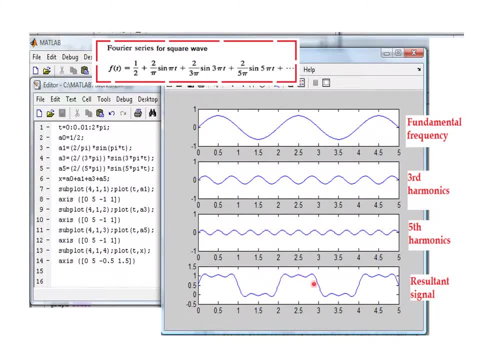 The wave shape is a V. This is a V. This is a V. So the wave shape is a V, This is a V, This is a V. wave shape is something like a square. it is not perfect as yet, because to make it perfect we need. 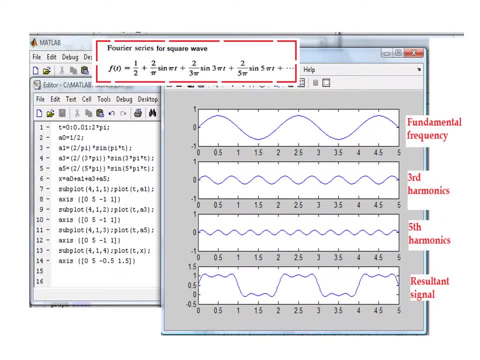 to add many more harmonics, at least 10 or 20 harmonics. so like, after third harmonics, fifth harmonics, then seventh harmonics, ninth harmonics, eleventh harmonics, like way you achieve perfection. but this is just to give an idea that the square wave is made up of combination of sine waves. 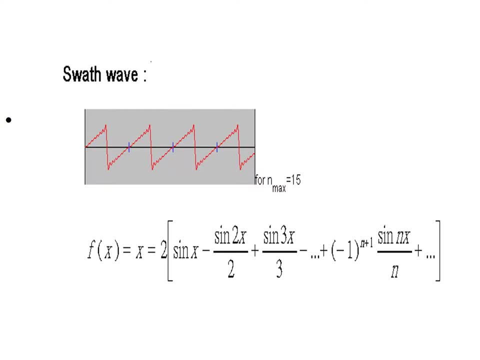 and similarly it can be shown that a sawtooth wave can also be constructed by various combination of sine waves. now in this case you can see sine x minus sine, twice x, that is the second harmonics, plus sine 3x, third harmonics. learn like this: by combining you can get a sawtooth wave. 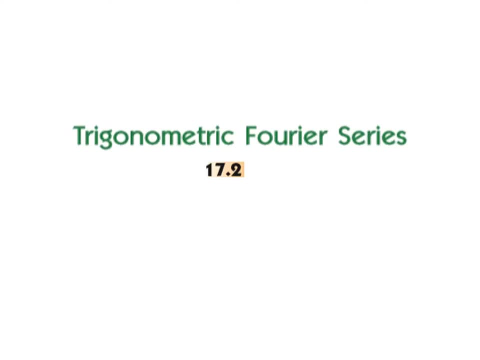 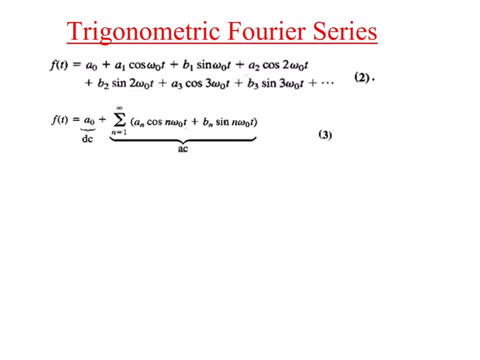 now the main topic, that is, the trigonometric fourier series. so the function that we saw earlier, same function. it is represented by various combination of sine and cosine signals. now this can also be written in a simplified form. we write this as the dc component, as it is. 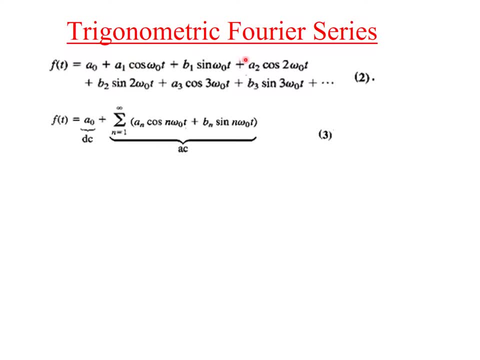 and then we add all the terms, cosine terms like a1 cos omega t, a2 cos omega t, a3 cos omega t, and we call them a n cos n, omega n, not t. and similarly we combine all these terms of the sine terms and we call them b? n sine one omega t. and then we sum up: from n is equal to 1 to 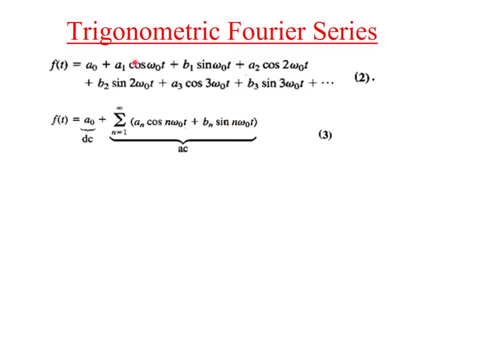 infinity. so these are the ac terms. so the same trigonometric function can also be written as in equation number three, Now omega naught. this one is the fundamental frequency, as we discussed, and any multiple is the harmonics. So if it is multiplied by n, this will be called nth. harmonics is: 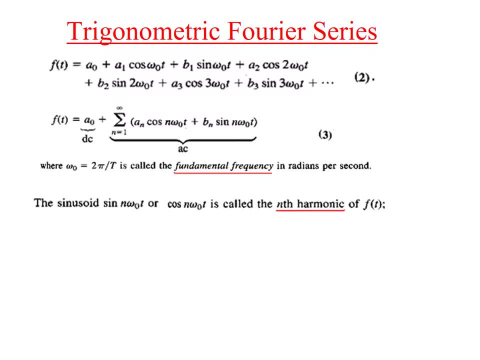 this multiplied by 2, that will be the second harmonics. multiplied by 3, it will be third harmonics, So three times the fundamental frequency. Third harmonics mean three times the fundamental frequency And the terms a, n and b n are called the Fourier coefficients. Basically, these represent the 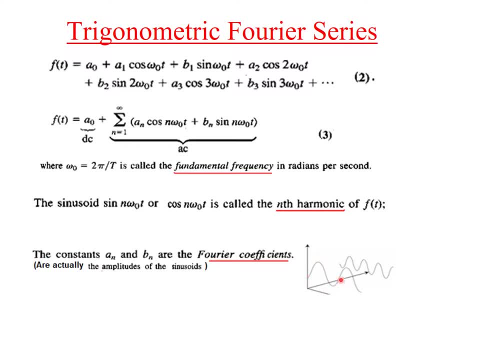 amplitude of the sign signal. So like, if this is one of the sign signals, this amplitude a1, this is another sign signal, sign signals, let us say its third harmonics or second harmonics, then the amplitude will be a2, but and they are generally known as the Fourier coefficients a, n and b? n. 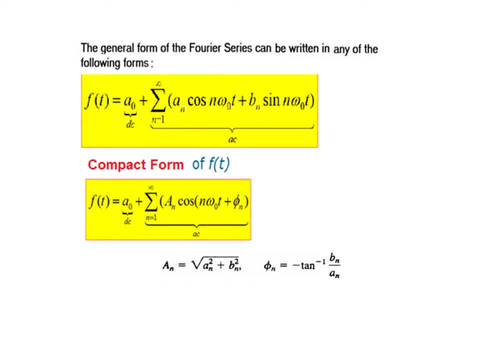 so this was the form that we saw in the last example. it could further be simplified in another compact form. so a naught remains like this, but this: these two can be added by this relation, that is, a capital, a n, cos n, omega t plus phi n, where a n. 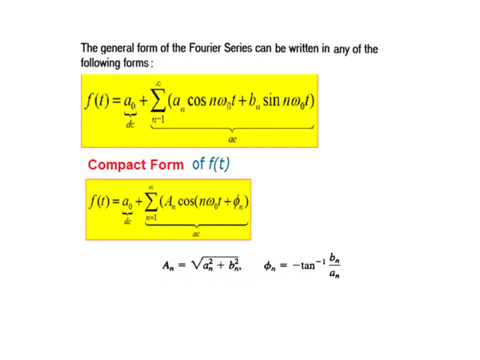 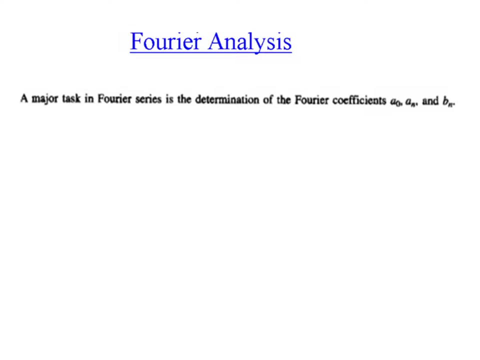 is small a n square plus small b n square under root. so that is the magnitude and phi is the phase angle and given by minus 10 inverse b n over a n. so this is another way of writing the same trigonometric signal. so what we need to do when we are trying to analyze is that we have to find these three. 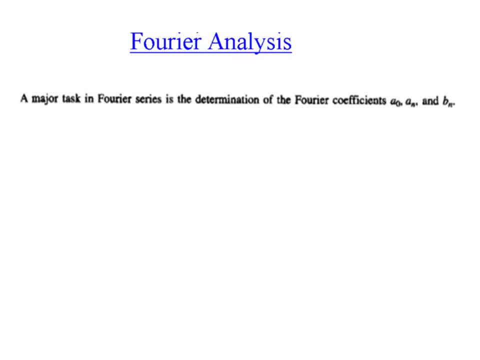 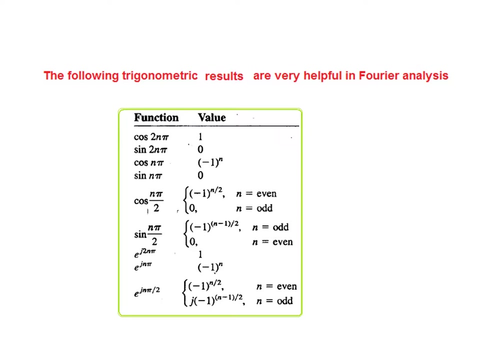 magnitudes a naught, a, n and b, n, and then we can put those values into the general equation given, so we get the complete answer. so the process of determining the coefficients are called Fourier analysis and, just for your reference, some of the trigonometric functions that are very helpful: 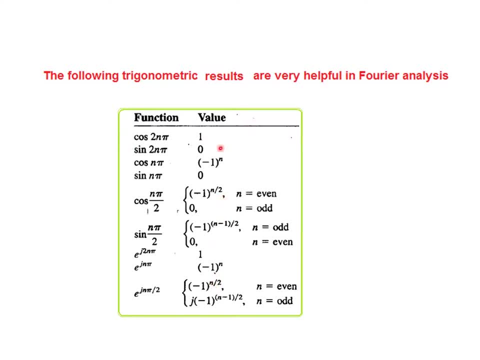 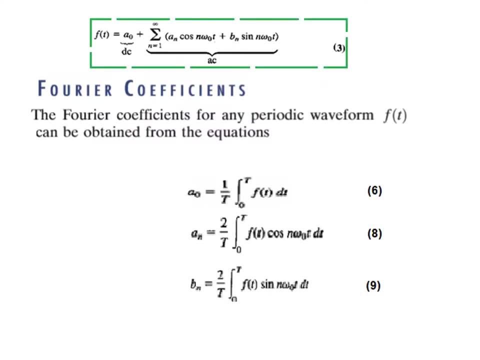 in solving fourier equations. you can just go through this and have a look. so the three coefficients that we need to find out are given by these three formulas. I have not gone into the derivation, but you can look into any book and you can find the derivation. The first one is A naught. the DC value is 1 over. 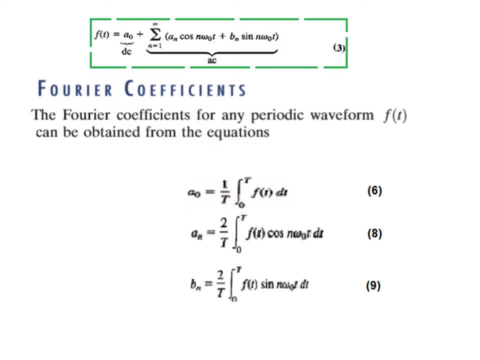 t integral of from 0 to 2 ft dt. So this is actually the equation of average value. if you recall, from instantaneous value, to get average value we use this formula, but this we will use for A naught. Similarly, to find A n, we will use this formula: 2 over t. 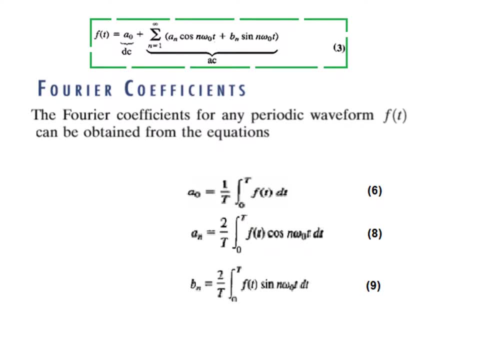 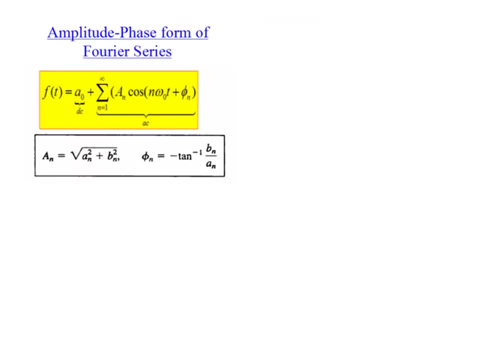 integral ft, cos, n, omega, t, dt, and to find B, n, we will use this formula And if you want to find the amplitude and phase spectrum, then we have, we can use this formula. here we need to find the value of A, n and value of angle so we can plot And the plot of the 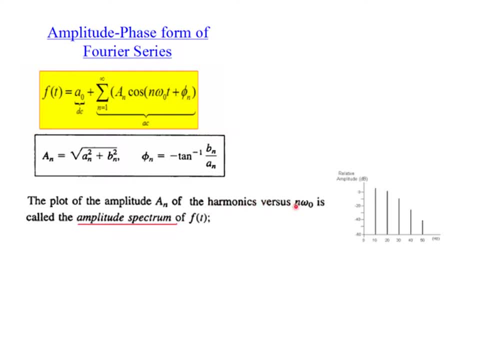 amplitude A, n. this, one of the harmonics versus frequency, is called the amplitude spectrum. So you can actually see now in this example you can see the various amplitude of various frequencies as shown here. So as the frequency is increasing, the signal amplitude is decreasing. 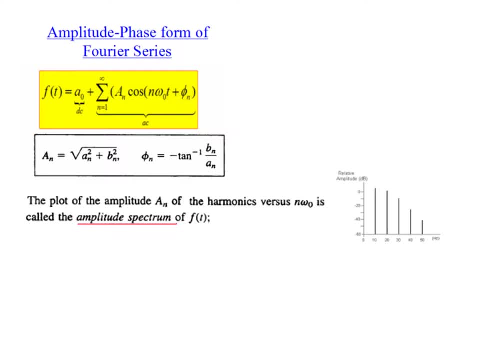 So this representation is called the amplitude spectrum. amplitude spectrum And similarly the representation of phase, this one in terms of frequency, so various angles. this is called the phase spectrum, And the combination of two is called the frequency spectrum of this signal. 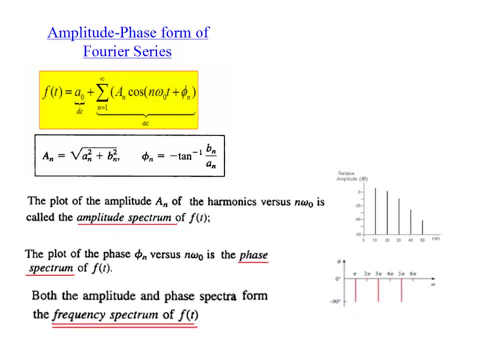 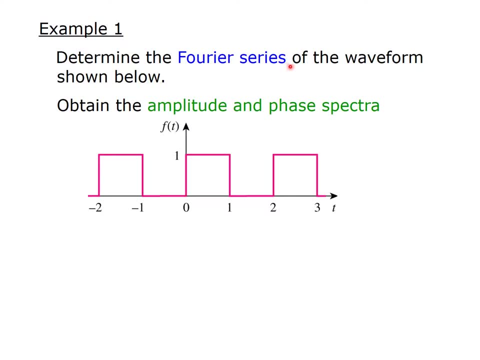 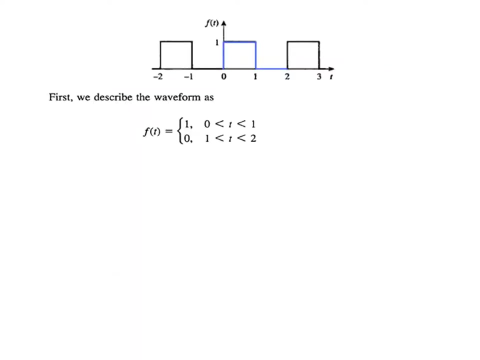 Now let us solve an example. you have to determine the Fourier series of the waveform given below, and also we have to plot the amplitude and phase spectra. So for the first one, let us define this. we will use this equation to find the three values a0,, an and bn. Before finding the values, we have to define the. 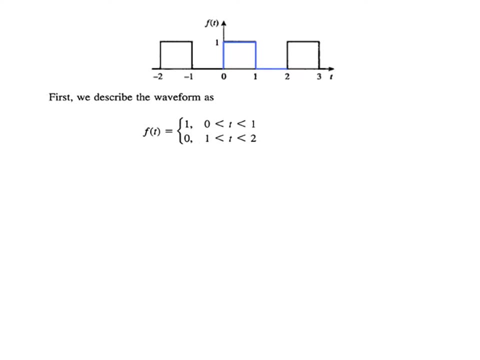 signal we take one period. So if we look at this signal, this period is from here to here. So from zero to two is one time period and the amplitude from zero to one is one. So we will write it like this: then the function t is equal to one, for t is equal to zero, to. 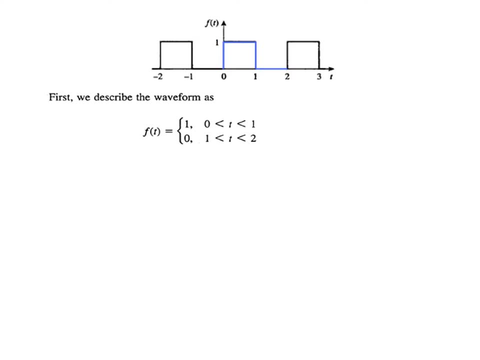 one and its value is zero from one to two. So we write it. zero from t is equal to one. Did you understand? Yes, So we will write it so that we have to find the three values equal to 1 to 2.. So this is how we define the function over one time period. 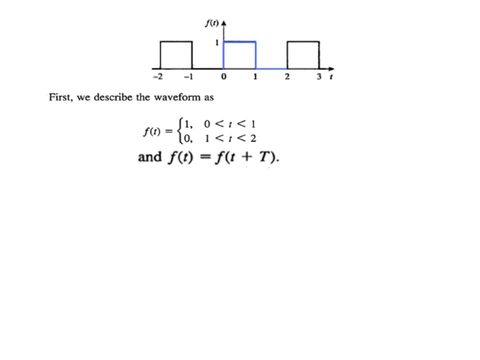 And this way of writing implies that the signal is periodic. So f t is equal to f t plus t means the signal is periodic. Also, from here we can see that since t is 2, therefore omega naught, we know the formula: omega naught is 2 pi over t, and putting the value of t 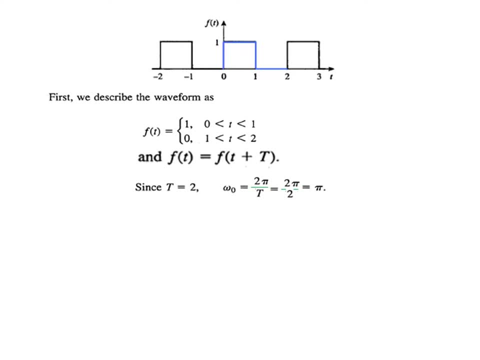 it is 2, pi over 2, and that means omega naught is pi in this case. Now, with this information, we go on to the, to finding A naught. So this was the equation for A naught. Now we put, the value of t is equal to 2.. So it is 1 over 2, and then we 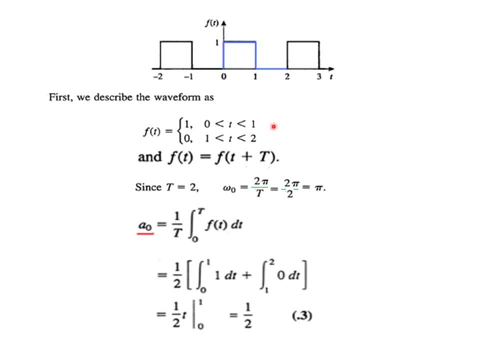 integrate Now, since the signal is divided into two parts, So we will have to integrate it into two parts. from 0 to 1, its value is 1.. So we write 1 d t plus from 1 to 2 its value. 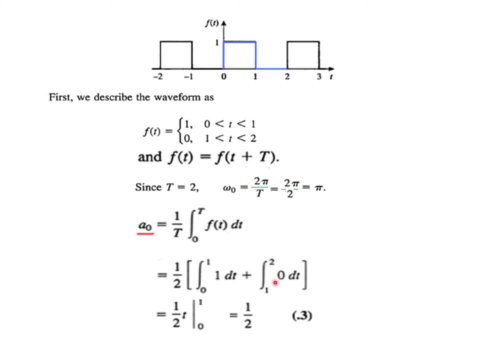 is 2.. So we write 0 d t and then this term becomes 0 integral of 1. d t is t over the limit from 0 to 1, and putting the value of 1 minus 0. We get the result as half. So this is how we find the first term, the dc term, or A naught. 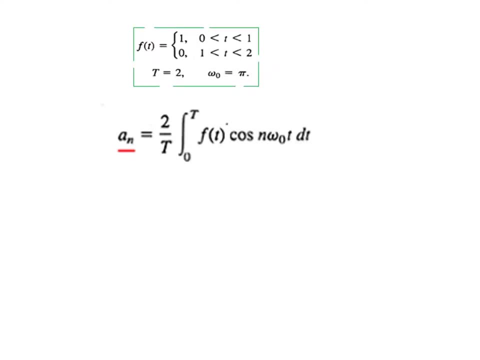 term. Now let us go to the second term, Same data that we got earlier. Now this was the equation: 2 over t, integral 0 to t, f t across and omega t. Now let us put in the values. So again for t we put 2, f, t from 0 to 1 was 1, so this will become 1 cos and then 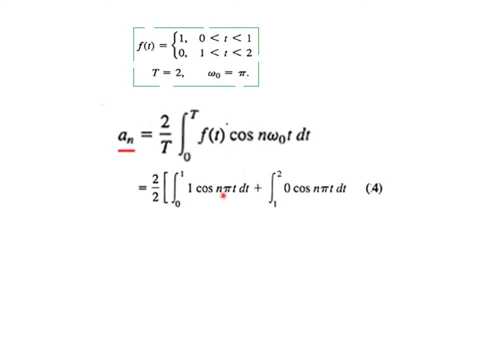 omega naught is pi, so it is n pi t dt. So that is for the first part, and in the second part it is 0 multiplied by cos n pi dt, because the signal f t is 0. And we know that the integral of cos is sin. So sin n t divided by whatever was the multiple. 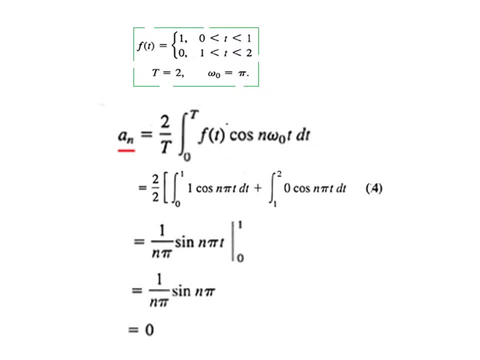 of t, so divided by 1 over n pi, and this 2 over 2 becomes 1.. So this is the integral of cos n pi, dt result. and then we put the limits from 0 to 1, and for t is equal to 1 and for t is equal. 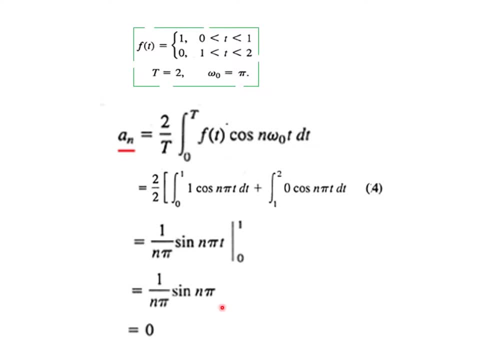 to 0. putting the values, we get this as the final answer. And now, since it is sin n pi, irrespective of the value of 1, the value will be 0, because we know that sin pi is 0 because sin 0 is 0. so, whether it is on the positive side or 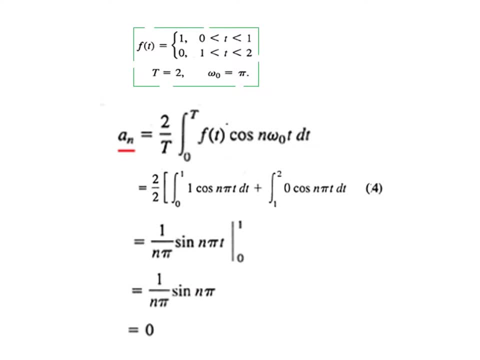 negative side, this value will be 0. that means a n is equal to 0.. Now the second part, b n, the formula 2, by t 0 to t, f t. now this case it is sin n, omega t. again we put the values now. 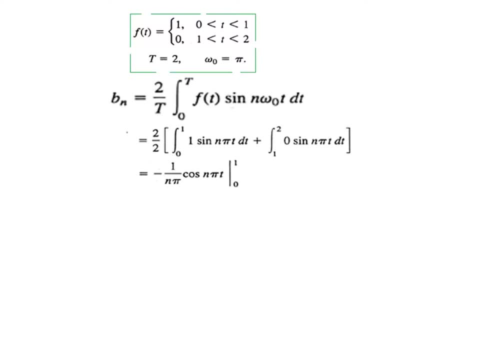 So 2 over 2, 0 to 1: 1 sin n pi t and 1 to 2: 0 sin n pi t. this term becomes 0, and integral of sin is minus cos n pi t divided by n pi, and then we put the value of 0 and 1.. 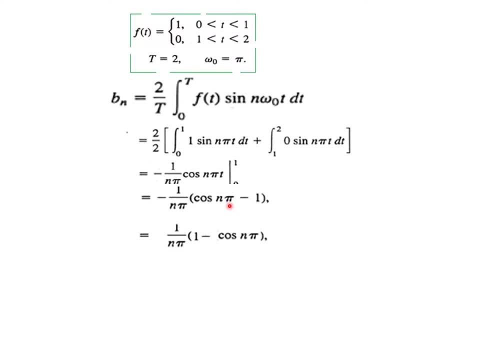 So this becomes cos n pi t, So sin n pi t. when we put 1 and when we put 0, this becomes 0. so cos 0 is equal to 1 and this can be rewritten as minus sign multiplying. so this will come: first plus and then minus. 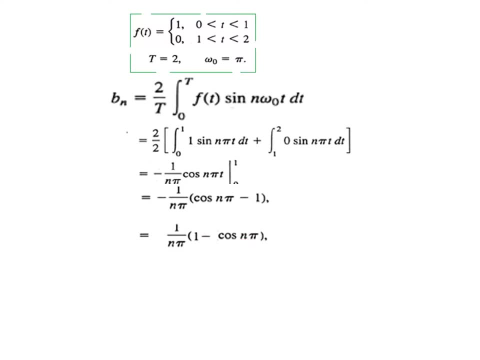 cos omega t. And now some trick that we have to keep in mind, Because the value of cos n pi Changes with the value of n. so we know that cos pi is minus 1, cos 2 pi is plus 1. so we write that as minus 1 to the power n. 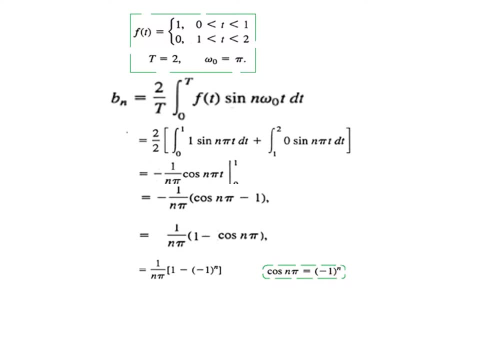 So cos n pi is equal to minus 1 power n, and if you put n is equal to 1.. So this will become cos pi, this will become minus 1.. So cos pi is minus 1.. Now, if you put n is equal to 2,, then this: 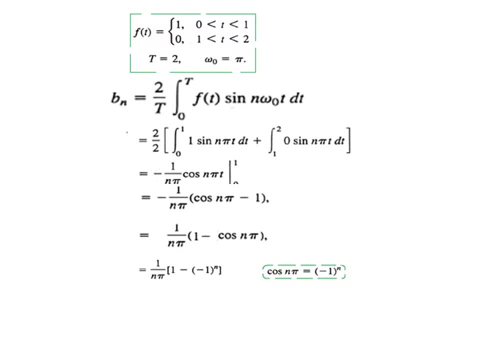 will become minus 1 square, that is positive 1 and cos 2 pi we know is. it makes one round and then comes to 0 and cos 0 is 1.. So this is positive 1.. Similarly, if n is 3, it will. 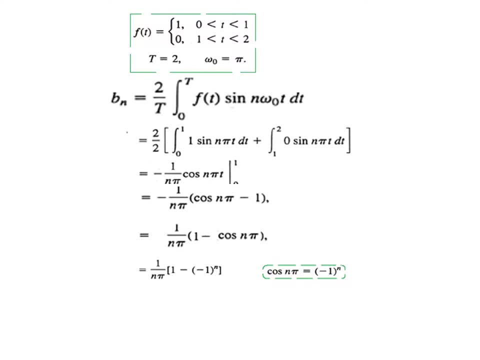 be minus. if n is 4, it will be plus. So that is how we write to represent this. So, instead of cos n- pi now, we write minus 1 power n Now, as we, as we discussed that, the value 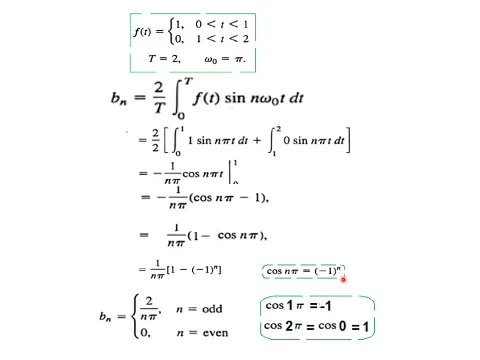 of cos depends whether n is odd or n is even. So when it is odd, it is. this value is minus 1.. When it is even, its value is plus 1.. That is why this whole result will be written in a manner to represent these two parameters, So like: when this becomes, this becomes minus. 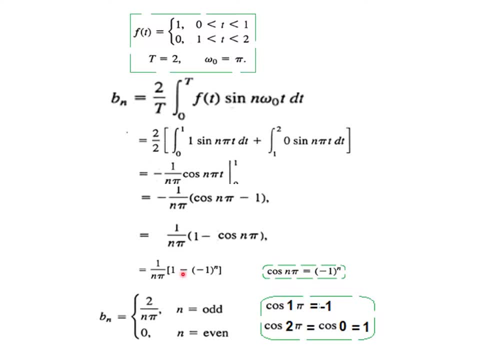 1, then minus and minus plus, So this will become 2.. So it will become 2 over n pi, And when this becomes minus 1, when n is odd, So for all n is equal toodd values, this will. 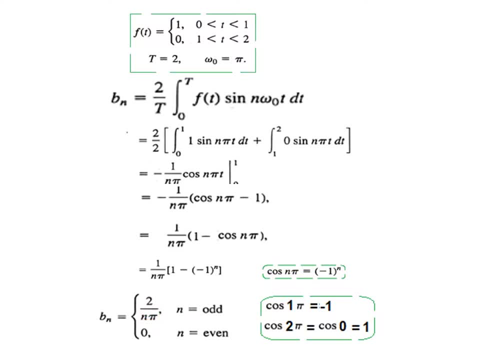 be the value of b, n, but when n is even, this minus 1 square will become 1, and 1 minus 1 will become 0. So the answer will become 0.. So these are the 2 valuesthat we get for. 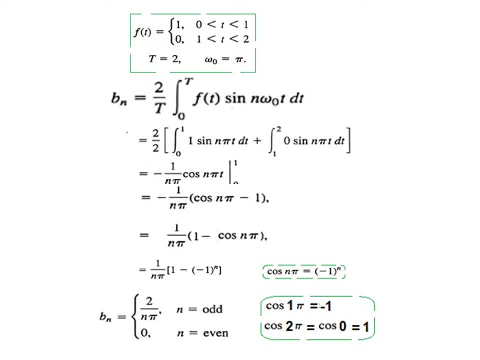 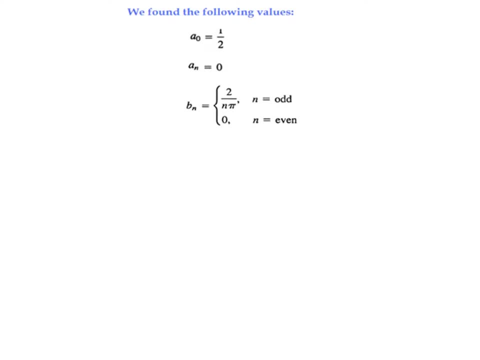 n is odd or n is even. So we found these 3 values and now we can write them in theto find the main function. This was the equation for the functions, and now we start putting the values. this was 1 over 2. All the cosine terms gone, because 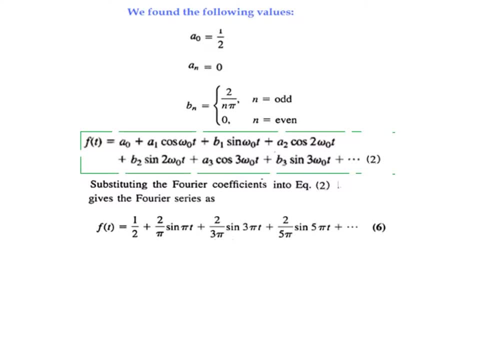 A n is 0, that means a 1 is 0, a 2 is 0, a 3 is 0.. So the cosine terms goes, and now we are left with the sine terms. So 2 pi sine pi t and then 2 over 3 pi sine 3, pi by t and. 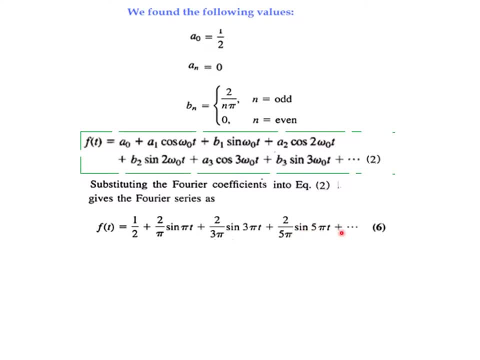 2 over 5, sine 5, pi by t. So all the sine terms remains. but if you look carefully, we do not have sine 2, but we have sine 3, and that is this thing: that when n is even b, n becomes 0. So that is why the even terms of the sine. 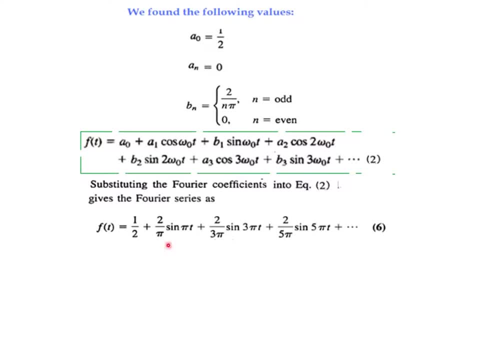 are also 0. So we have the odd time, odd frequencies of sine remaining. So I hope this gives you an idea as to how to find the coefficients and how to find the final Fourier series equation. and we can manipulate, we can just take 2 over pi common. 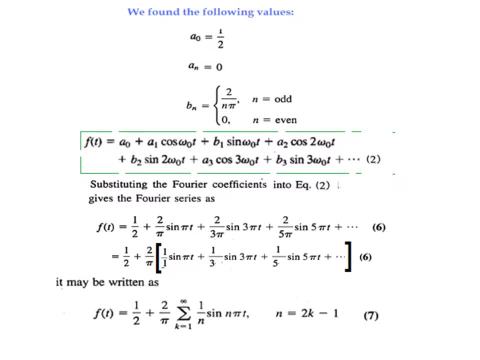 then we can further simplify your compact form this: 2 over pi, and this whole thing can be written as 1 over n, sine n, pi, t, where n is 2k minus 1.. Now, what is this? Why we are writing it like this? Because we know that here n is only odd number, not even. 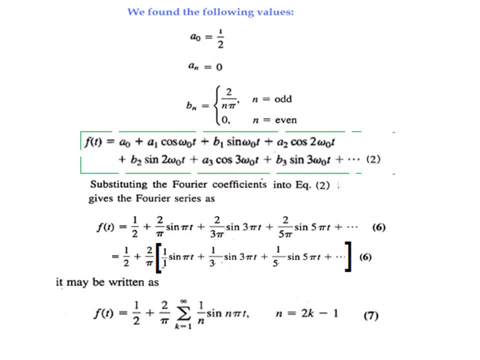 So if we write it, n is equal to 1 to infinity, then n would be 1, and n would be 2, and n would be 3, so that this relation will not be valid. So to make this relation valid, that only the 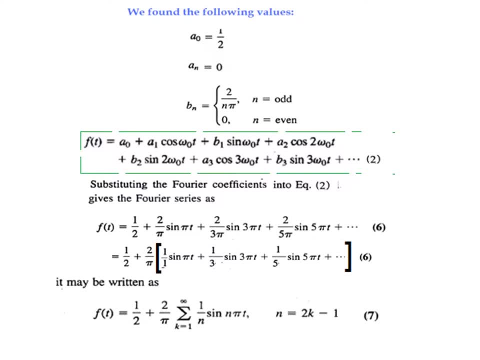 odd numbers come. we defined another variable, and that is k. So n is actually 2k minus 1.. So what does this mean? So we can write it like this. So what does this imply? If k is 1, like here, if k is 1, then this will become 2 minus 1,. 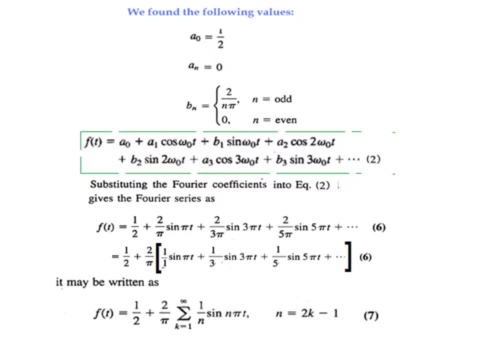 so that is equal to 1,, so n is odd. Now, if k is 2,, this becomes 2 to the 4 minus 1, 3,, so n is still odd. If k is 3, then 3 to the 6 minus 1, n is 5, so it is still odd. So 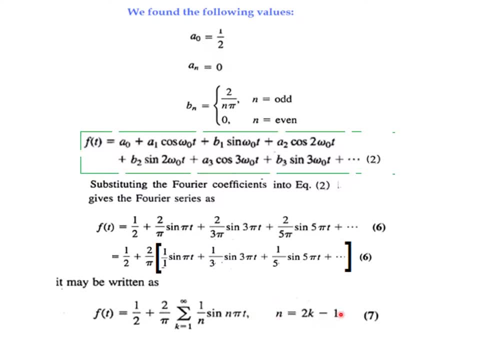 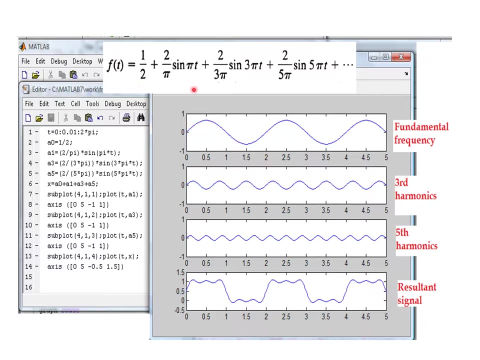 this is the way we represent or make sure that n is only odd number. So we will do another example, but before that, this is the same thing that we explained earlier. This is the equation now that we have got, and if we plot this equation, this represent a. 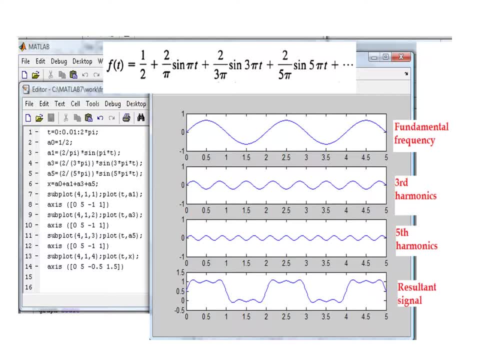 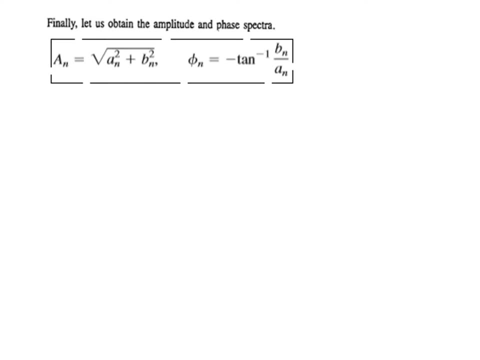 squarish wave shape. So actually, we started from the square wave shape and we found that a square wave shape, as represented by this, is a way that, because of❤️ the change in today's Euh, if I am placing here a flat surface, 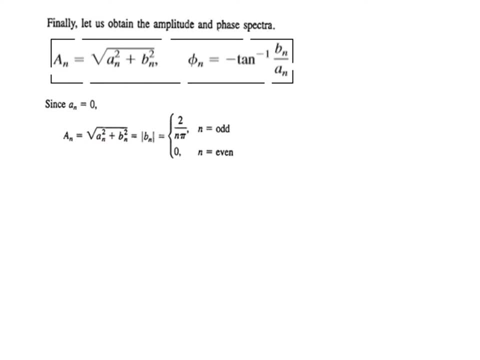 Then when I am using the horizon nosso温 angle, then I represent convey terms, For example, that if I am applying in ku igual to 30 stage, HTTP, tucked the surface and leave just this 1, k plus providingkelijk cliche. tightly dreamed les will be got, But worked on theência of this creepingopersfeed the hearth, and only naturally there is a case because 2d will decreased in the come up, which no debate. output and onion is 1.. Now the second part of the question, that is, we had to plot this spectra. the amplitude is spectra and the phase spectra. Now this was the relation for the amplitude and this is for the phase. So let us put the values in this. So let us put zetoklone and the change in the exaggerated nadaglak. 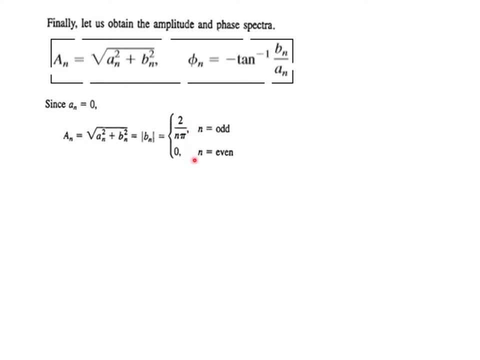 actually b? n, and so this was the value of b? n, and that becomes the value of the amplitude spectra. and now this is the plot, this is the plot of the, if you keep on putting the values of n here. so in the first case, when n is 1, this will be 2 over pi, so this is 2 over. 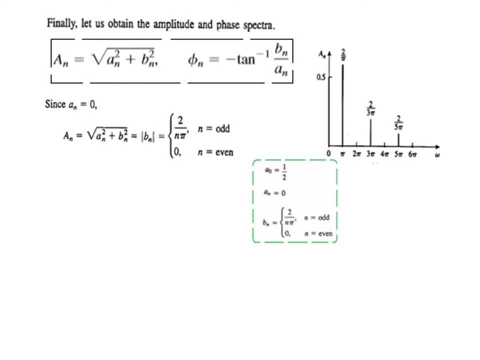 pi, and when n is 3, because n 2 does not exist, when n is 3, then this will become 2 over 3 pi. so this is 2 over 3 pi. it is at odd 3 pi. then you will have a value at 5 pi. whose value? 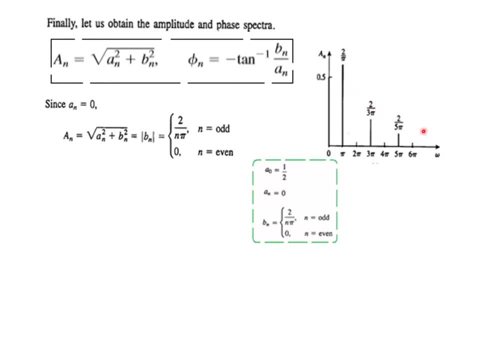 will be still lesser. So the amplitude spectra is this. So the amplitude spectra is this. The amplitude spectra is this: The amplitude spectra is: this is gradually decreasing. Also, you can see, this is the DC component, or A naught value. So 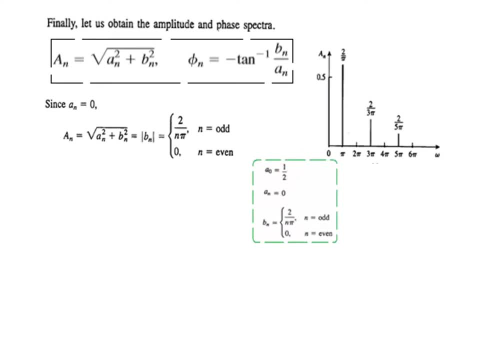 we found A naught to be 1 over 2.. So this is 1 over 2 or 0.5.. This is how we plot the amplitude spectra. And now let us see the phase. This was the equation for phase and putting the. 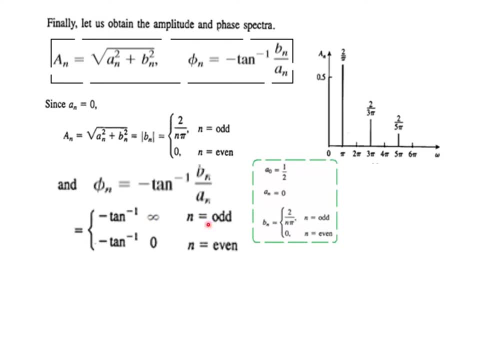 values when n is odd. So when n is odd, we have Bn2n, pi, 2n, pi and an is 0. So anything divided by 0 will make it infinity. so this is minus 10 inverse infinity, And when it is even. 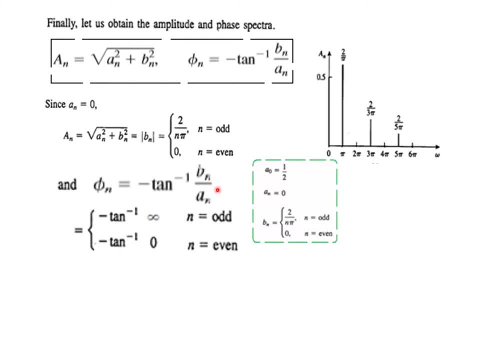 then it is 0.. 0 over 0, or we can say they are equal and therefore the result is 0 when n is even. So how do we plot this? Okay, from here, we convert them in terms of degrees, So we know. 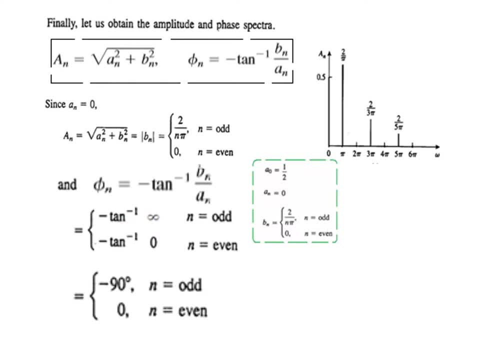 that 1090 is infinite. So that means the angle is minus 90 and 10: 0 is 0. So the angle is 0.. So when n is odd, it is minus 90, and when n is even, the angle is 0.. So we plot it like this: